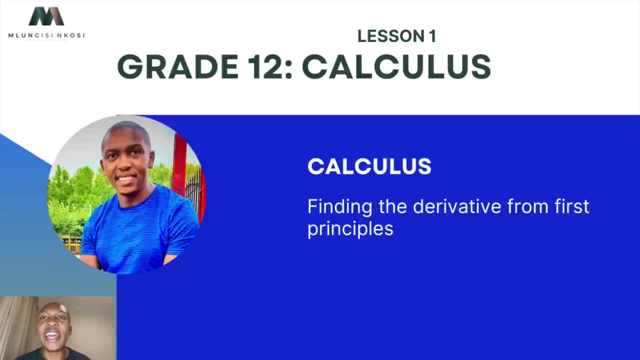 All right, and so today we are starting on a new topic, and that is calculus. I'm excited to start this one and hopefully you'll stay for the rest of the series. okay, I'll try to develop it, you know, such that you are able to understand it fully. 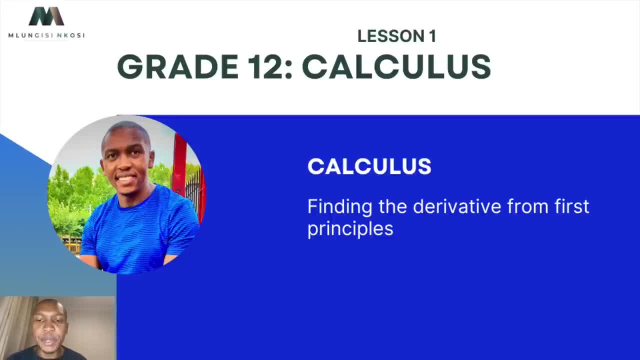 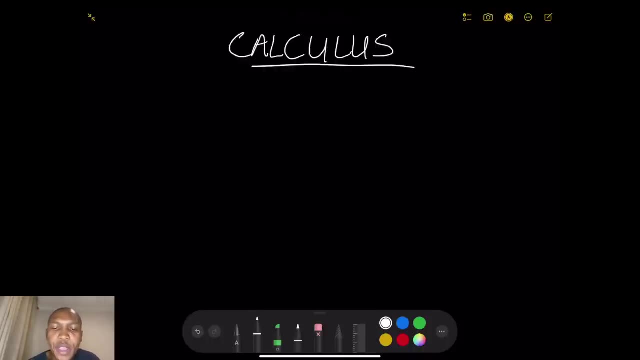 Today we're going to be exploring just the concept of first principles, or of differentiating using first principles, But first of all, what I want us to do. all right, let's begin here, When we're talking about differentiation, okay, so let's take just for argument's sake, 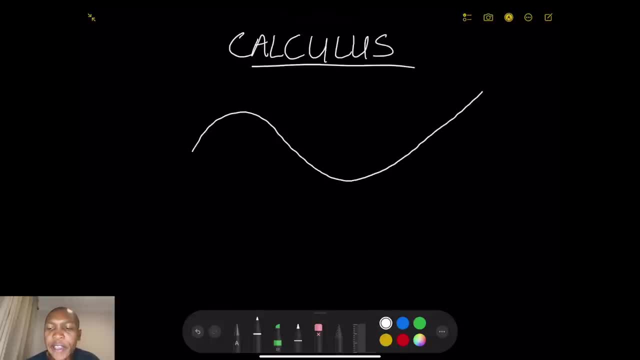 if we've got a curved function- okay, something that looks like this- it may look differently, All right. so let's say, there's our x-axis and our y-axis, So there's x and there's y over there, All right? so when we look at this particular function, 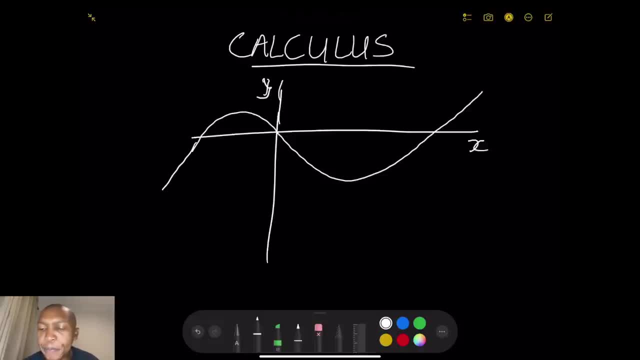 so we can get a gradient between two points. Let's just take, say, maybe that point and that point over there, right? So if we took the gradient between two points, what we end up with is a secant, If you look at that. so what a secant is? it's a line that cuts. 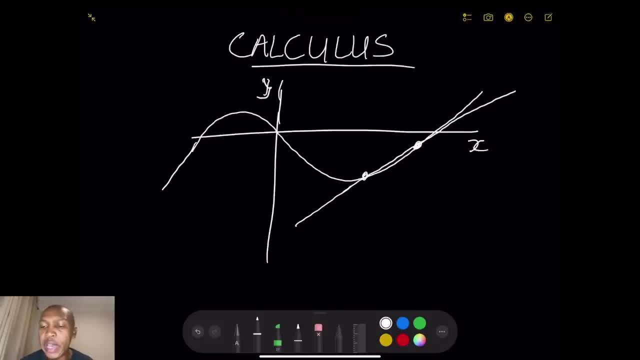 you know, into two or more points on a function. So if we decided, okay, we're going to call that point, let's say x and that point over there, that would be x plus h. So h would be the difference between the two points. So if we take that point over there, that would be x plus h. So if we take 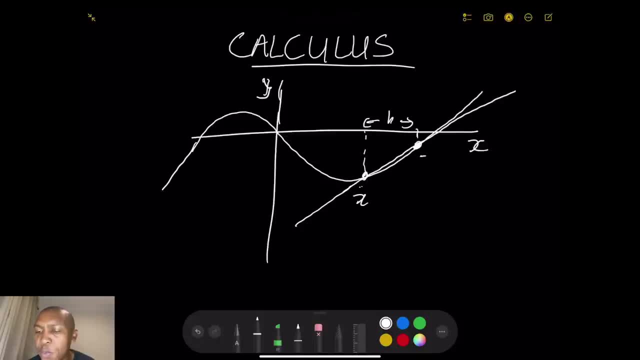 that point over there, that would be x plus h. So h would be the difference between the two points, So such that this would be x plus h. Now of course, the corresponding y value. let's call it fx, if the function here is f of x, right, So that means the corresponding y value here. 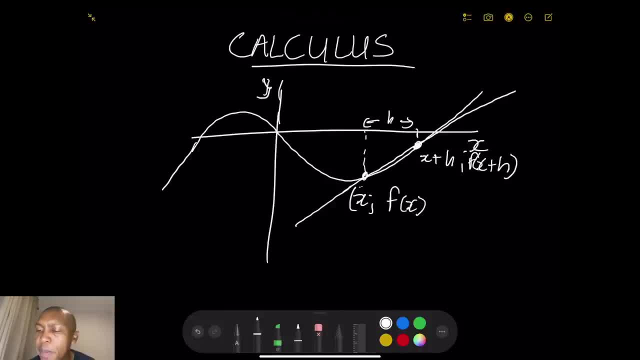 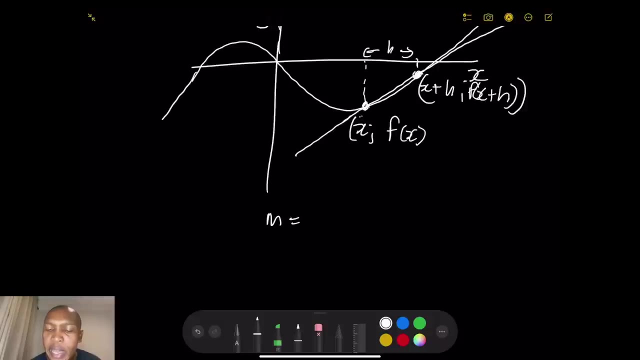 would be f of x plus h, okay. Now the problem is that if we look at those two points, what we get- okay, Remember, whenever you take the gradient m, that would be the change in y over the change in x. So what you get is f of x plus h, right, Minus f of x. okay, Divided by. 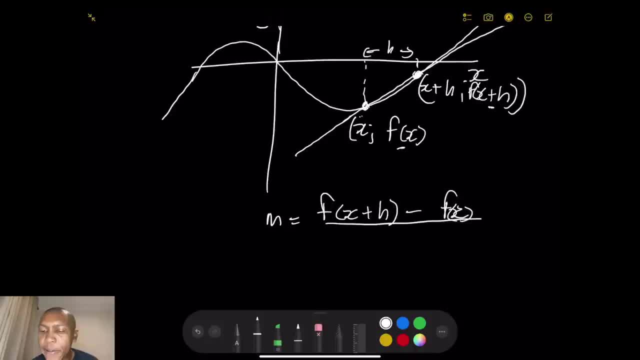 so that's change in y. So take the y's okay Divided by change in x. of course that will be f. I mean x plus h, So that's change in y. So take the y's okay Divided by change in x. 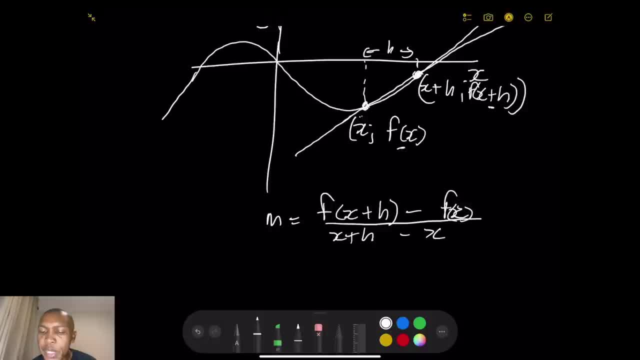 h minus x in this particular case. Now, when you take the gradient, what you end up with is what we call the average gradient. okay, Why? Because that's not the actual. Remember, the gradient keeps changing between those two points. The gradient keeps. 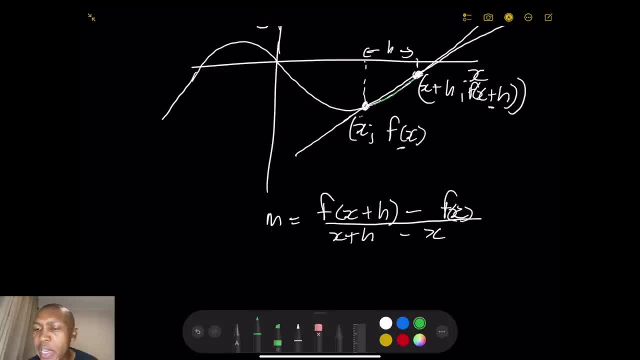 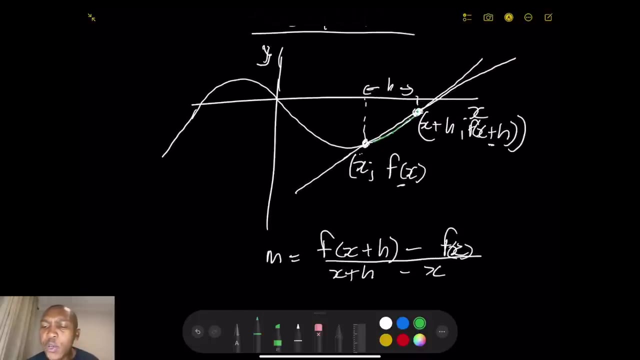 changing. in that particular case, It is not the actual gradient. Now, what can we do to actually change the gradient? Well, we can do this by taking the gradient. okay, So we can take the gradient at a particular point. We use the same principle and we say, well, what if we try to make? 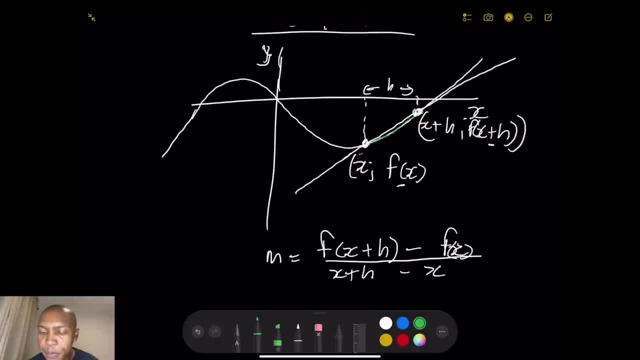 the value of h as small as possible, such that if I keep making h as small as possible- I'm going to try- and if the value of h is smaller, then what happens is I now start moving more from a secant and I keep doing that. 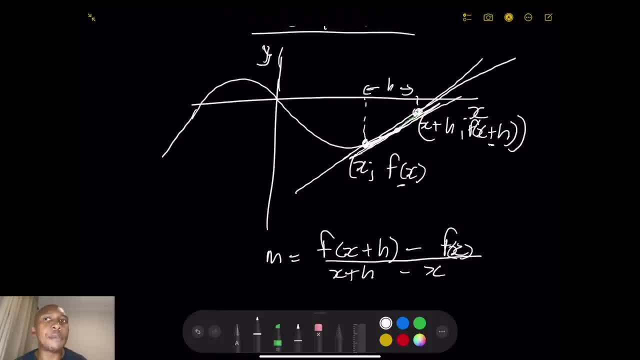 Until I get to a tangent. Now, remember what is a tangent? It's a line that touches, you know a function once, or it's a line that, whether it's a circle or whether it's a graph, whether it's a- 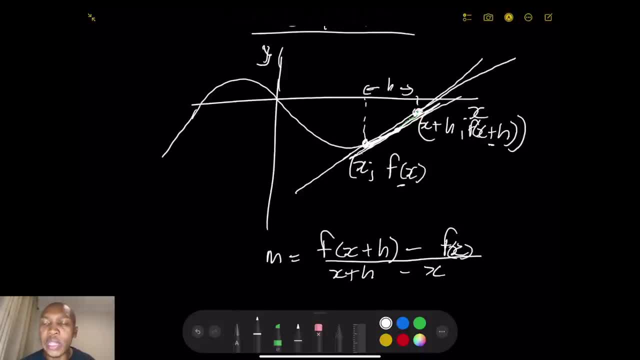 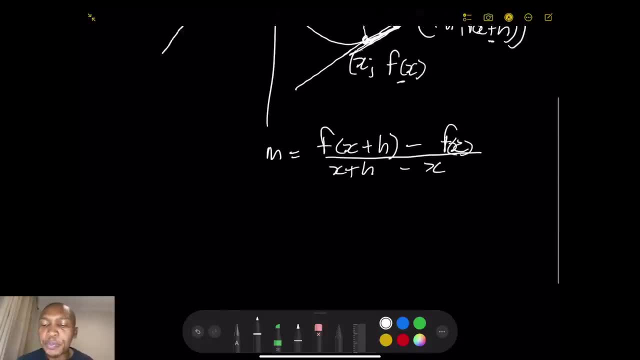 curve. whatever the case is, it's a line that only touches once. So you get to a point where you've got a tangent. okay, And that is why we're going to actually explain something just now, that when we deal with calculus- okay, Now note, whenever I'm asked in any graph to get f of, let's say our- 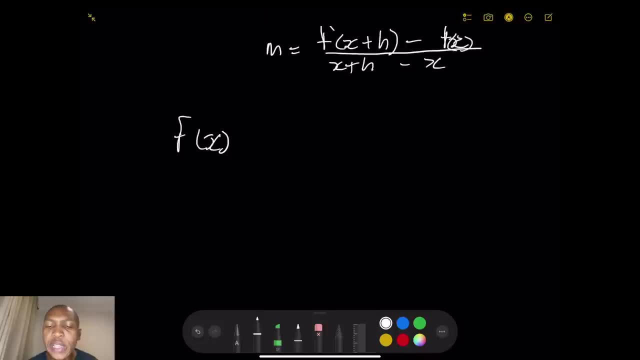 graph is f of x. for argument's sake, right Now, when they ask me to get what is f at 4,, what is that? This simply means? this is the y value at x is equals to 4, right, So this would be the y value. 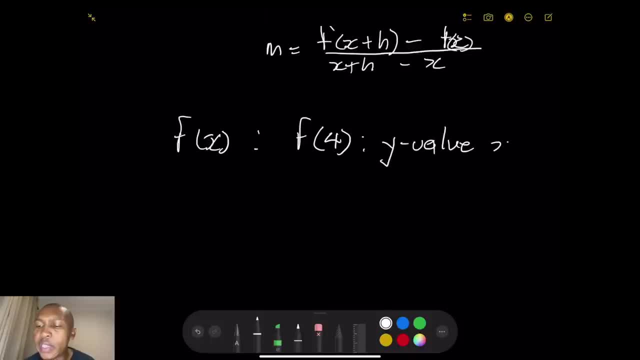 Right Where x is equal to 4, right. But what does it mean when I'm getting f dash of 4?? And, by the way, f prime, that's the symbol that we use for, you know, the derivative right. So what does it? 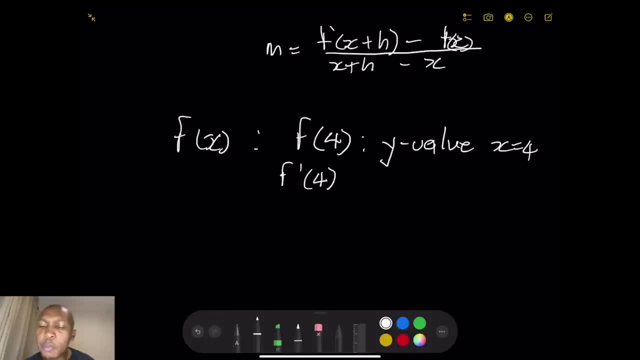 mean when I get f dash 4?? This would be now- please, I want you to listen carefully- right? So this would be f dash of 4.. And, by the way, f prime- that's the symbol that we use for you know. 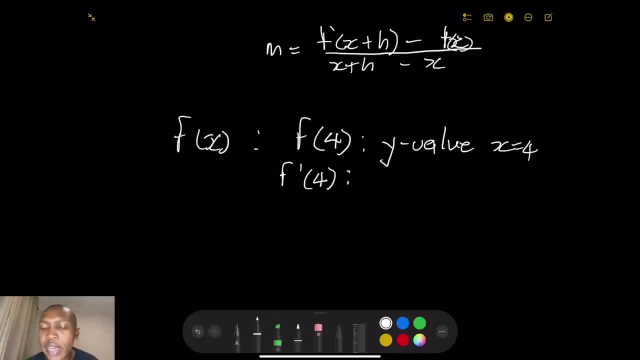 the derivative at x is equals to 4.. But what it simply means is that this is the gradient of the tangent. gradient of the tangent at x is equal to 4, right. So in this case, what you're getting is it's the gradient of the tangent at x is equals to 4.. 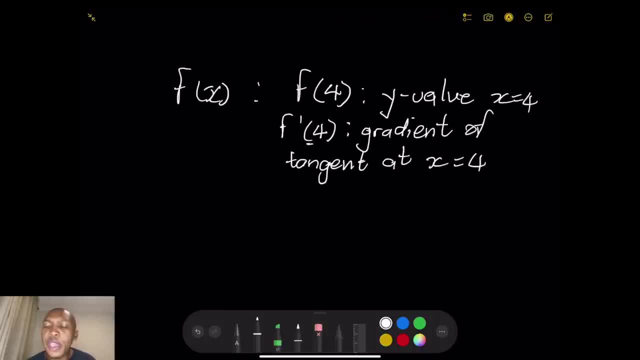 In this case, I want you to please note that once we start talking derivative, remember that we associate this with the gradient. okay, Right. So this is the gradient of the tangent at x is equals to 4.. Now we can do this in different ways. We're going to deal. 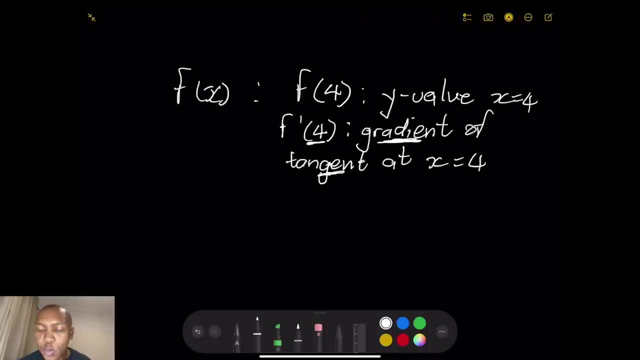 with differentiation a little bit later on. all right, But what I would like for us to do is explore what we're talking about here. So let's start with. the gradient of the tangent at x is equal to 4.. And, by the way, f- prime- that's the symbol that we use for you know. the gradient of the tangent at x is equal to 4.. So let's start with. the gradient of the tangent at x is equal to 4.. And, by the way, f prime, that's the symbol that we're talking about here When we're 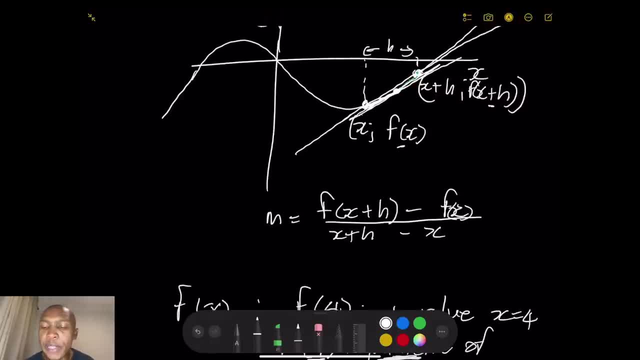 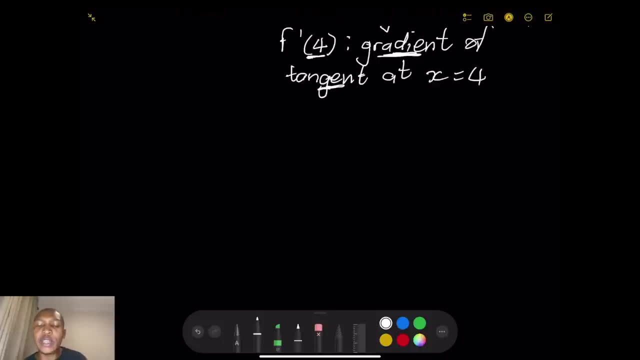 talking about, you know, taking the first principles right Now, in this case, what we do to get the derivative. remember, we said f dash. what it simply means is that you are taking the derivative. So what we simply say is that f dash of a function right would be equal to now. 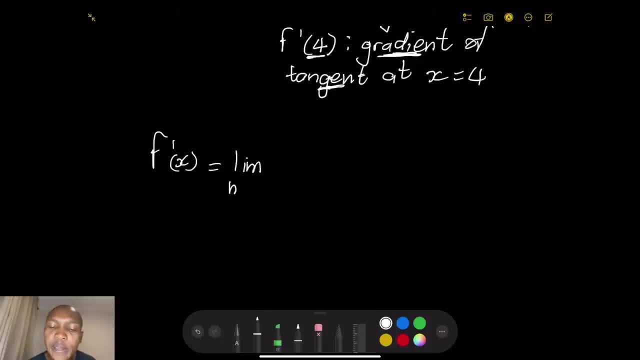 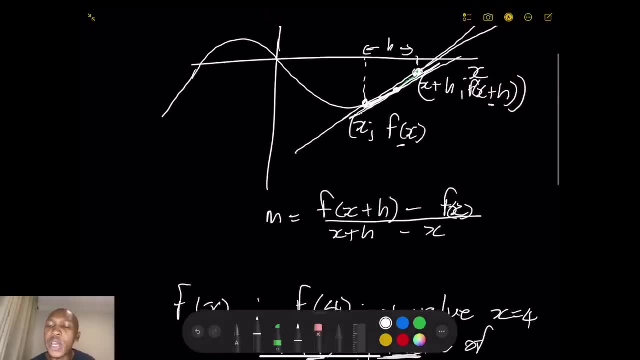 first of all, we say it's the limit, As h tends to zero. Now, if you remember what we said, we said h tends to zero. It means that we are trying to narrow that value of h to be smaller and smaller up until we move from it. 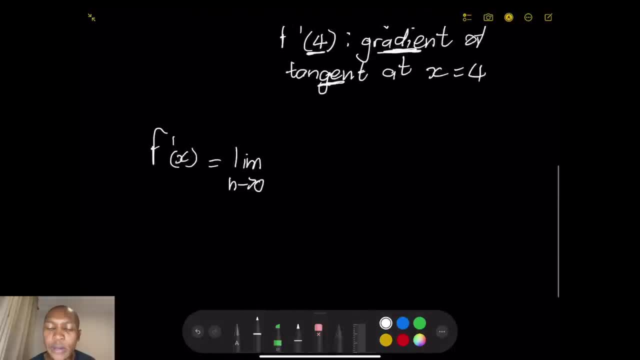 being a secant, to it being a tangent. okay, So we say it's the limit, as h tends to zero, of f of x plus h minus f of x divided by, in this case, divided by h. And remember how did we get that h? If you noticed, we would cancel that and we would have 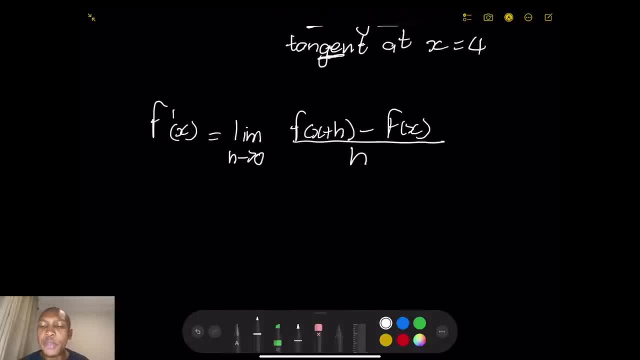 h over there right Now. so we're going to just explore a few examples where we are going to use, in this case, our first principles in order to find the derivative. Let's get into our first example, All right. So our first example says: determine f, dash x, the derivative. 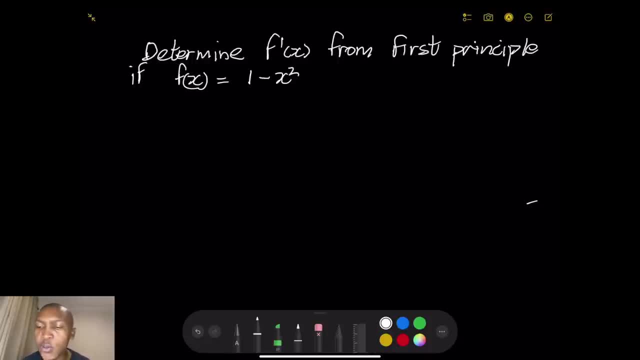 from first principles- And you need to look out for that word: from first principles. If they didn't say it, of course we can do it just the ordinary way And we'll discuss that a little later on. Right? So they said: from first principles: if f of x is 1 minus x, squared Now. 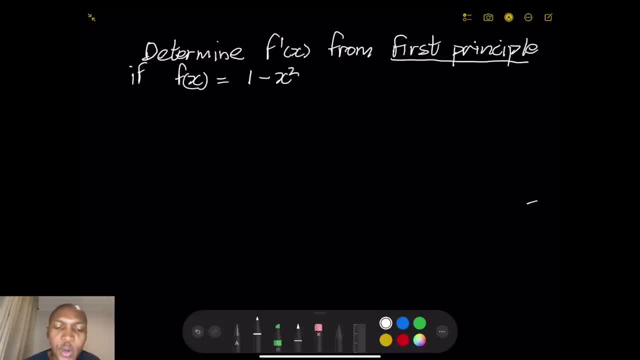 remember. so what we simply do in this case, we're going to remind ourselves: remember f dash x, in this case, would be equal to the limit Right, As h tends to 0.. Now, you do not remove this until you get to the point where you've just 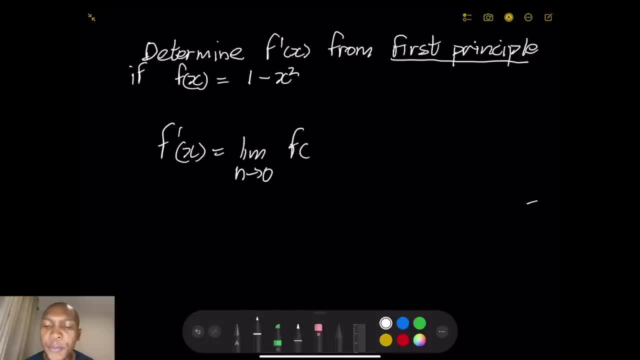 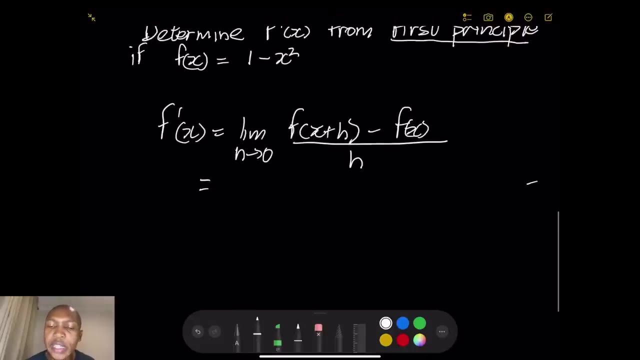 clarified everything, But we'll get to that in just a few, Right? So that's going to be x plus h minus f of x. okay, divided by h. Now, for as long as we are not substituting 0 for that h. 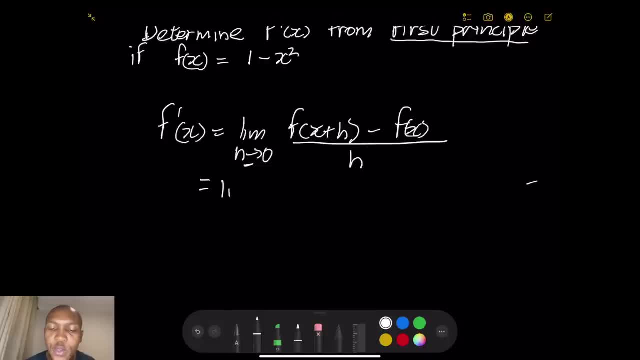 we are not removing this expression here, So this is going to be limit, as h tends to 0.. Okay, What is our f of x plus h? So it means that in your f of x equation, you are going to substitute x plus h everywhere that you see x. right? So this is going to be. 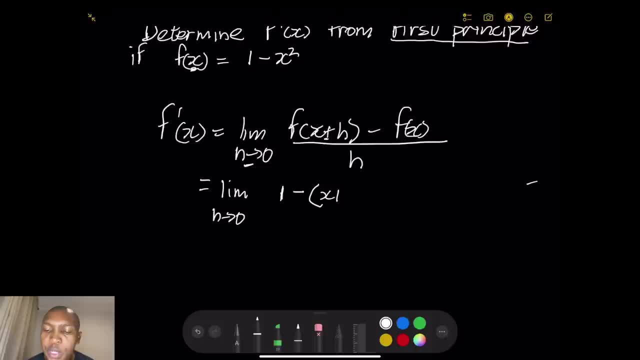 that's 1 minus where I see x, I'm going to put x plus h squared. Remember expression was 1 minus x, squared minus what is our f of x. Now, please remember to put that in a bracket. So that's 1 minus x squared. Okay, Divided by: 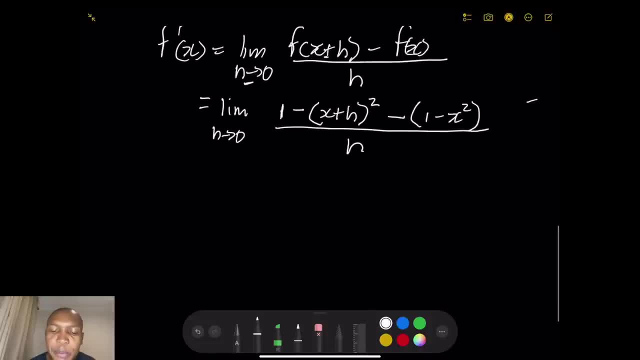 in this case, h. Now we're going to try and simplify everything until we get to a point where- remember, what we're trying to do is we need to finally remove that h in the denominator, because once we, you know, substitute for h is equal to 0, then what it simply means is that: 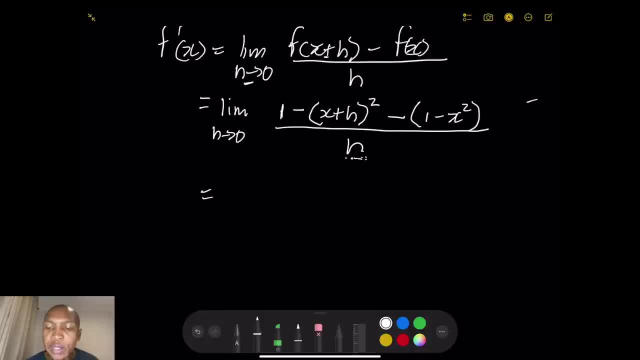 I mean, our solution becomes undefined, Right? So we're trying to get rid- that's what we're trying to ultimately do- get rid of that h in the denominator. So let's simplify. So remember, we don't remove this expression. 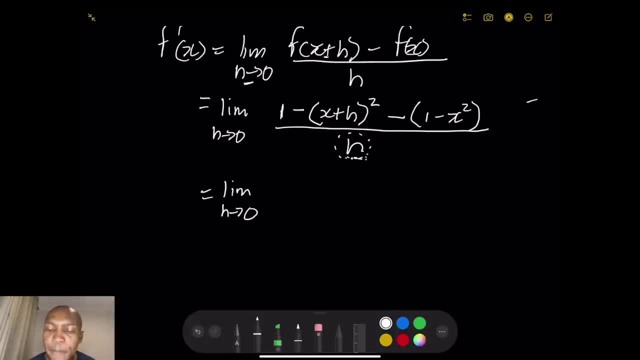 as long as we have not substituted right. So this is going to be 1 minus. Now let's try and expand this. So this is going to be x squared, all right, plus 2xh plus h squared, Okay, Right. And then, remember, this is going to be minus 1 plus. 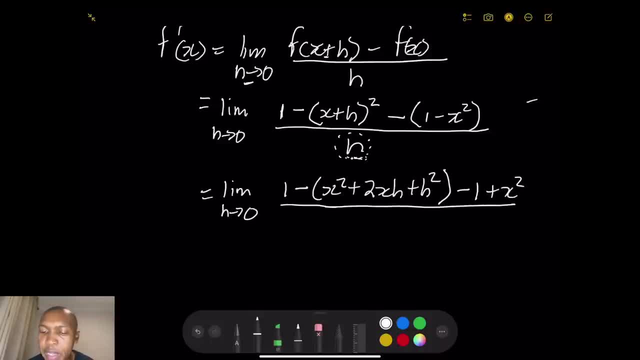 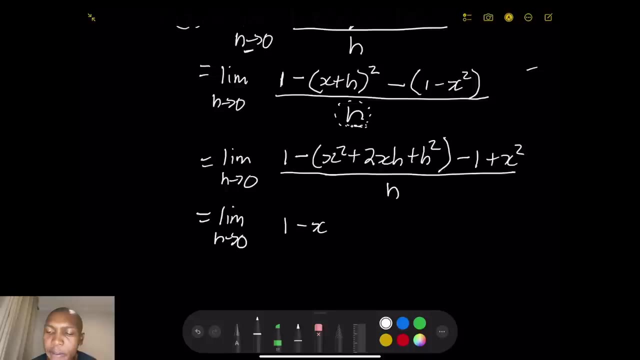 x squared divided by h. Okay, So we're still going to try and simplify. So this limit, as h tends to 0.. Remember, we have not yet substituted. So that's 1 minus x squared minus 2xh minus h squared minus 1 plus x squared divided by h. Now let's try and get rid of. 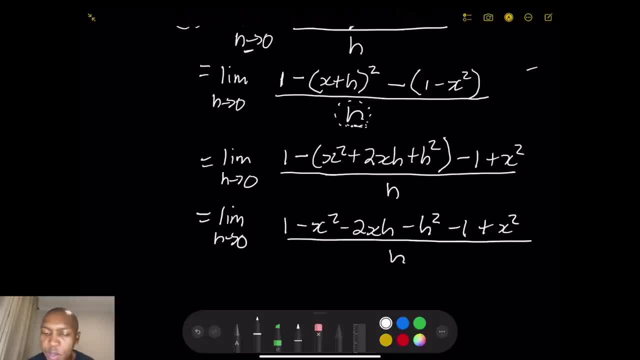 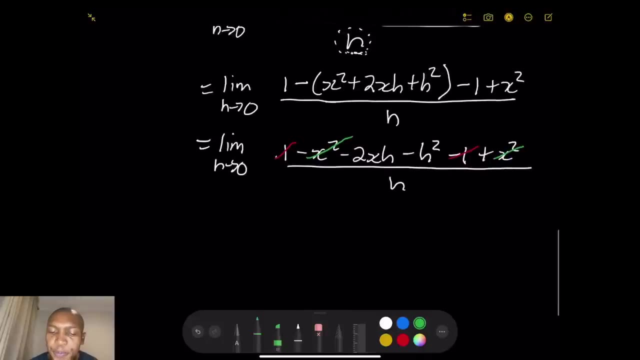 you know what we can get rid of? Okay, I see I've got a 1 and minus 1 there, so we can cancel those. Okay, I've got a minus x squared and a positive x squared there, All right. So in this case, what are we left with at the top Right? So you can. 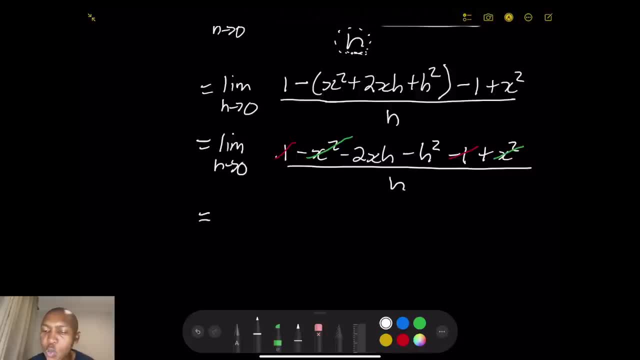 see we've got minus 2xh, minus h squared. So why don't we take out h as a common factor? So I'm going to take out h as a common factor there on those two, So that becomes minus 2x, minus h, right? 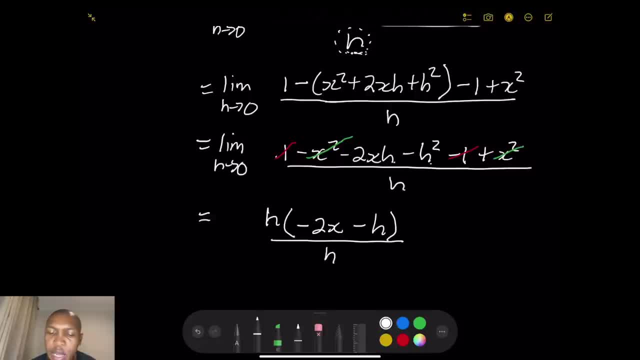 Okay, Divided by h. You see, now I'm violating my own rules. So limit as h tends to 0. Okay, So what do we do now? Do you see we can now get rid of that h that divided by that. Okay, Now. 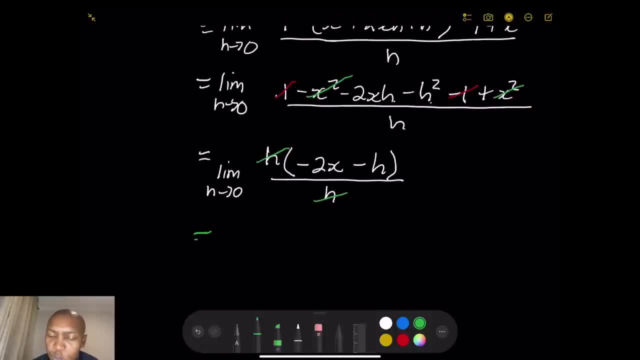 because we're getting to that point where we can substitute right, So we can substitute for that h there. So let us now substitute 0 for h, And I don't need to write that. I'm going to write this expression when I do that. So now I can say: well, this is 2 times sorry, minus 2x, rather. 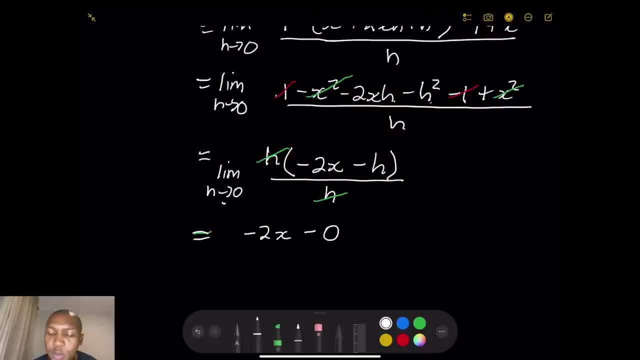 minus 0.. Okay, I'm substituting 0 for h, And what do I end up with? It means that I've got minus 2x And that is my derivative for that particular function that I had there. Okay, Right, Let's take another example. 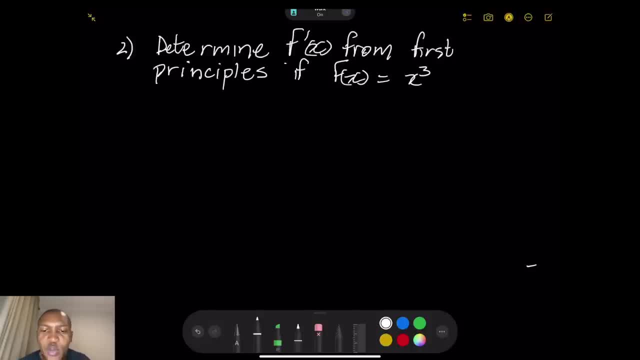 All right, Now let's look at the next one. Again, they say: determine the derivative f dash x from first principles if f of x is x cubed Right. So in this case again, we said, if you want to take the derivative, you're simply going to say: well, this is going to be limit, as h tends to 0.. 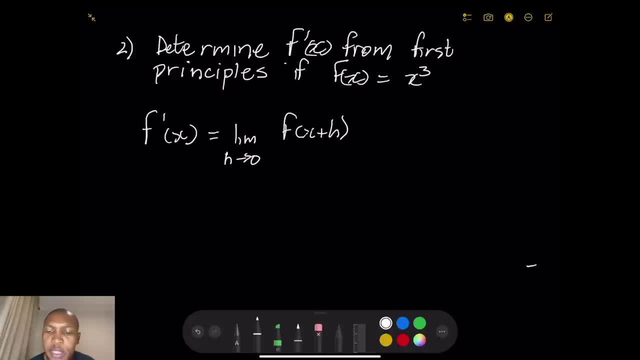 Okay, Of f of x plus h minus f of x divided by h. Now remember, what we always try to strive towards is just removing that h in the denominator. So let's do that, So let's try and expand this. So this is going to. 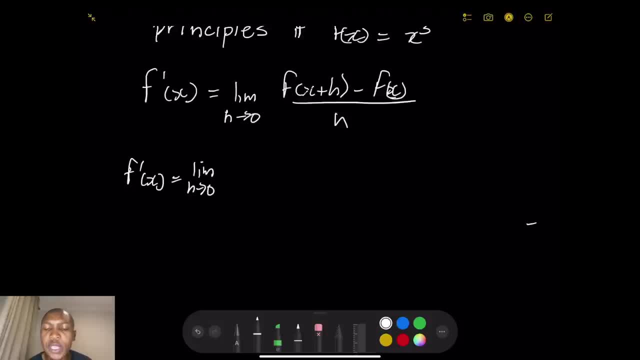 be limit, as h tends to 0. Remember, we don't remove this expression until we get to that point where we substitute for h, right, So x. f of x is x cubed. So this is going to be limit, as h tends to 0.. So this is going to be limit, as h tends to 0.. So this is going to be. 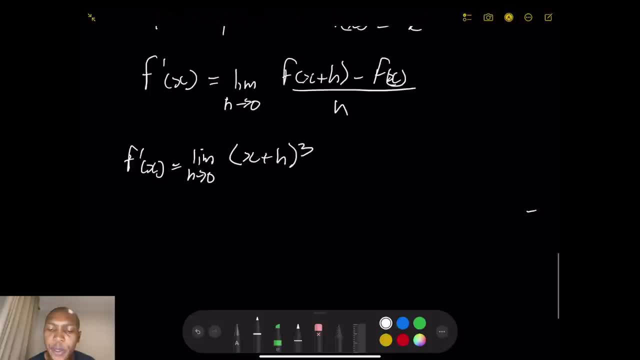 x plus h cubed. So everywhere we see x, we substitute with the x plus h in that case. So that's going to be minus. this was supposed to be x cubed, rather divided by h. Now what's left for us to do is to try and simplify this as much as possible. Okay, So this is going. 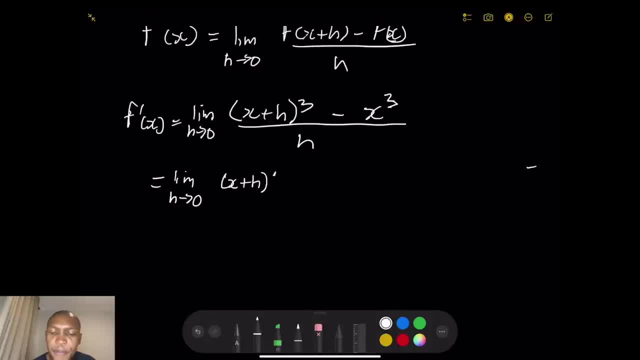 to be. this is the same as x plus h, into now x plus h squared. I'm just going to say this is x squared plus 2xh plus h squared minus x, cubed right All over h. Now, all I've just simply done there. 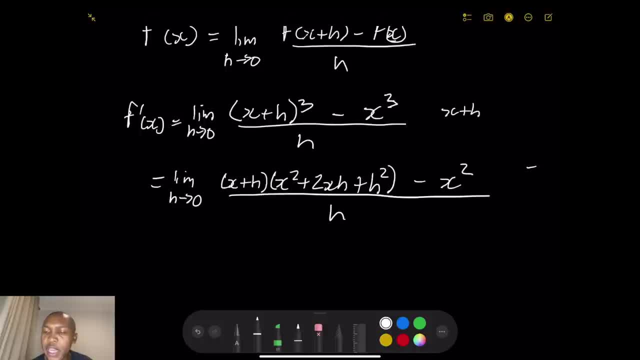 was just to take x plus h and x plus h squared, Right. We need to always find a way to make this as quick as possible, So I took x plus h squared and that resulted in x squared plus 2xh plus h squared. Okay, So yeah plus h squared in that. 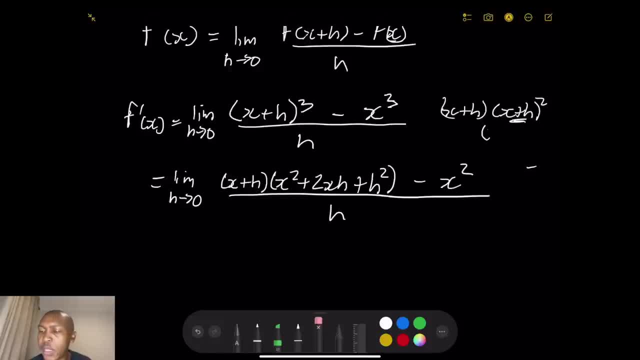 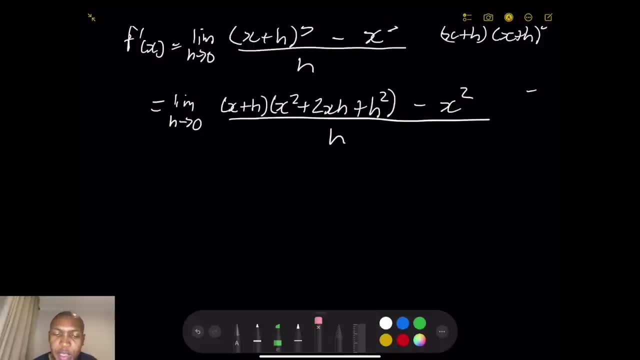 case, And that gave us the result that we got there right. So now what we're trying to do is, um, uh, get to that point where we can cancel, cancel the h, So at the end of the day, we've got limit, as h tends to zero. Okay, So now let's. 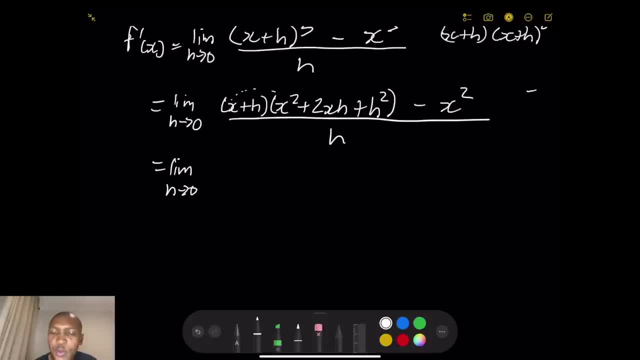 try and expand what we had there at the top. So we've got x times x squared. This is going to be x cubed. This is x multiplied by 2xh. That's going to be plus 2x squared h, And then x multiplied by. 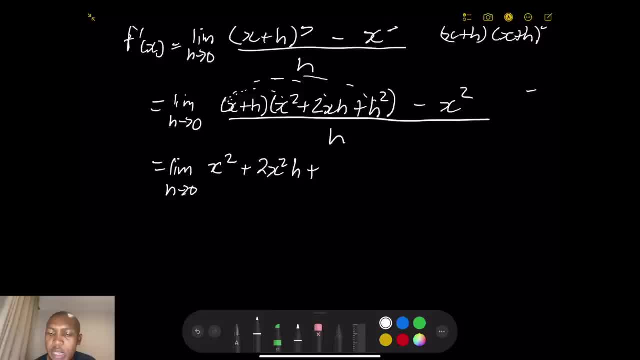 h squared. This is going to be plus x- h squared, right. And then let's get to the next one. So this is plus h. Okay, So let me just do it in the yellow. So we're going to have h times x squared. So this is going. 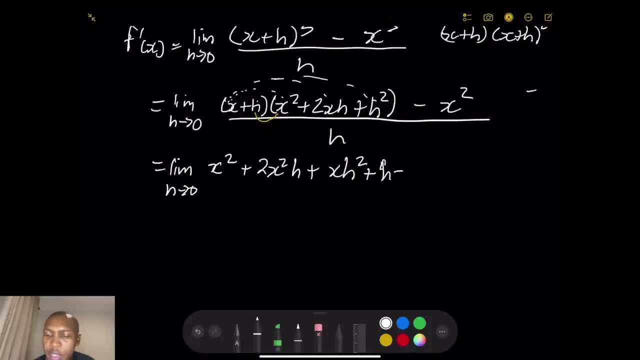 to be, uh, h x squared, Okay. And then we've got h multiplied by 2xh, okay, which is that one, and that's going to give us plus 2x h squared, plus 2x h squared. and then we've got h times h squared, which is plus h cubed. this is minus x squared, x cubed. 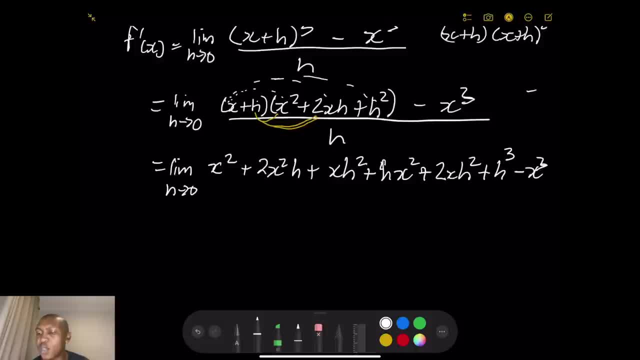 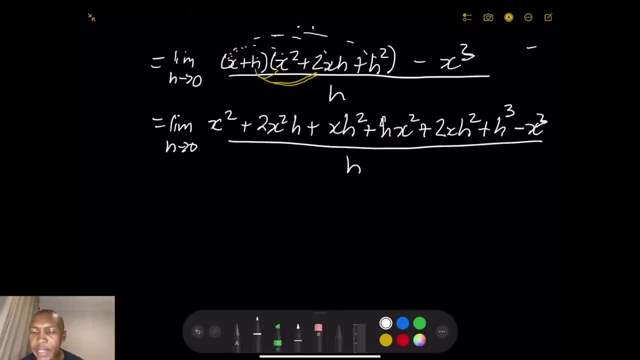 rather, why do i keep saying x, x squared. so this is minus x cubed, all right, divided by h. okay, so now, uh, let's see if, uh, in fact, first of all, that should have been x cubed as well and not x squared. okay, let's see if i got everything else right, okay, right, so now, uh, we know its limit. 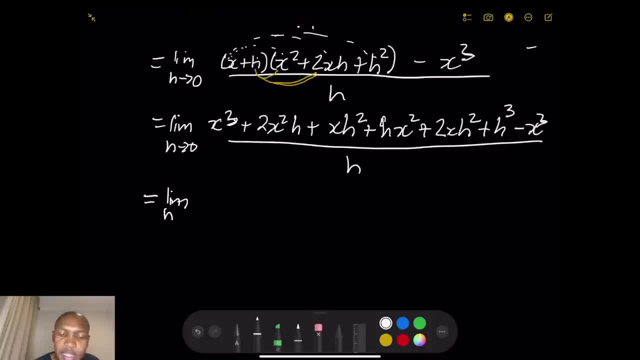 uh, limit as h 10 to zero. again, remember, you do not remove this until you have substituted, okay. so let's try getting rid of what we can. so we know that goes with that guy, okay, and um, which other one? okay, uh. so what we can do, uh, so we've got h x h squared, h x squared. 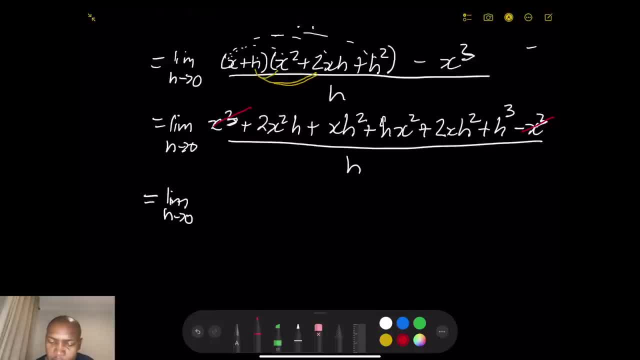 to x. okay. so i see that we've got, uh, some common factors there and you've got an x squared term there and another x squared term there. okay, so i am going to- and i've got an x term here, i'm gonna do it in yellow- and another x term. uh, yeah, another x term there. so let's try and. 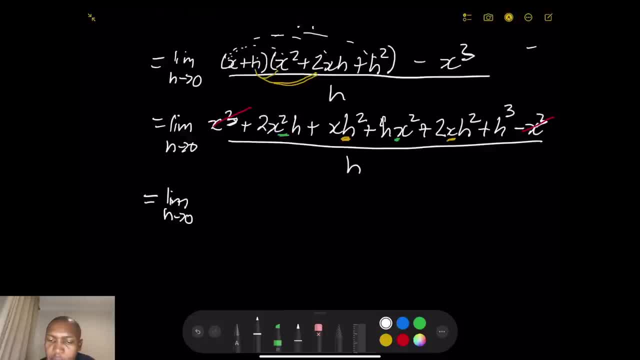 simplify that. so this is going to be: x squared and another x squared term there, and another x term there and another x term there. okay, so this is going to be: uh, two x x squared, h, or two h x squared, it doesn't really matter. so this is going to simply be plus that other one in green. so this: 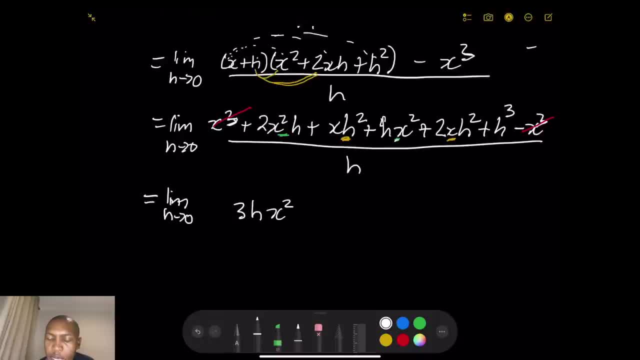 is going to be three h x squared, right, and then i'm going to also be adding those x terms as well. okay, so this is going to be uh, plus okay, another x h squared, two x h squared, so this is going to be plus three x h squared. or you can say two h squared, x, okay, and then so i've, i'm done with those ones. 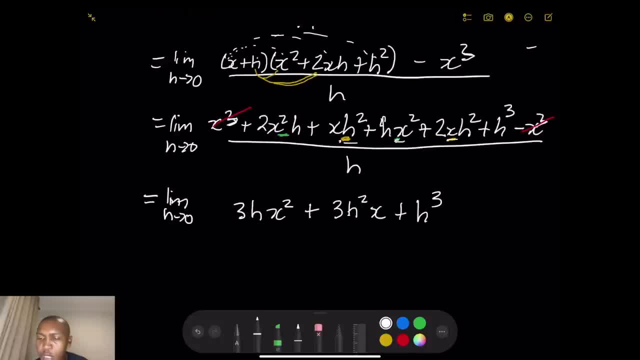 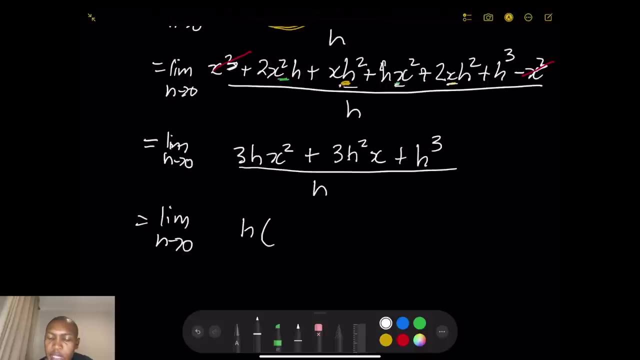 and then i've got plus h cubed, okay, right, and all of that divided by h. and what can we do now? we can now obviously take out h as a common factor. okay, so if i take out h as a common factor, i'm left with three x squared plus, uh, three h. 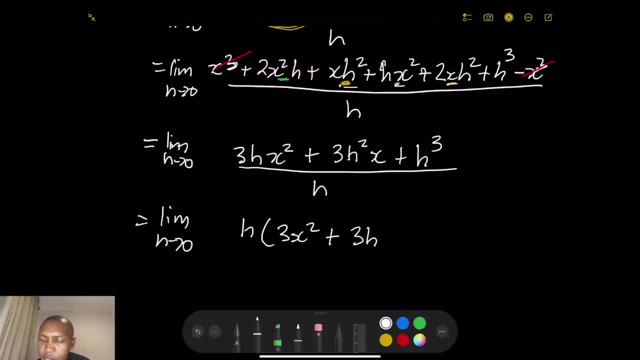 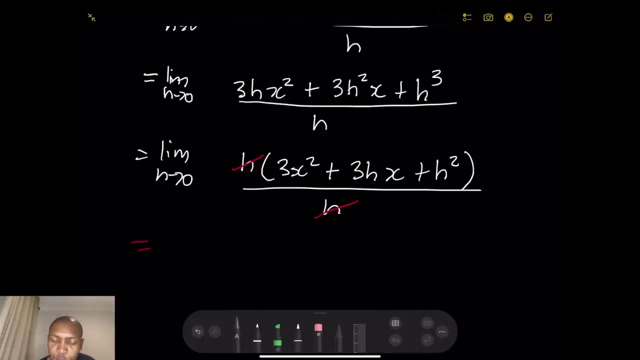 um, yeah, three h x plus h squared, okay, right, and in this case, divided by h. what can i do? i can actually cancel that h there. now we can substitute for zero. okay, so we can substitute: h is zero, so in this case i've got: okay, three x squared, okay, plus three. 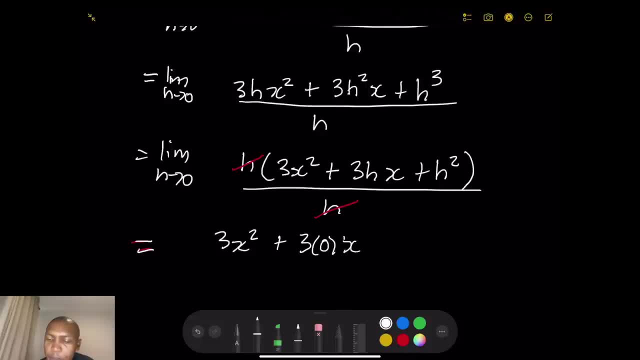 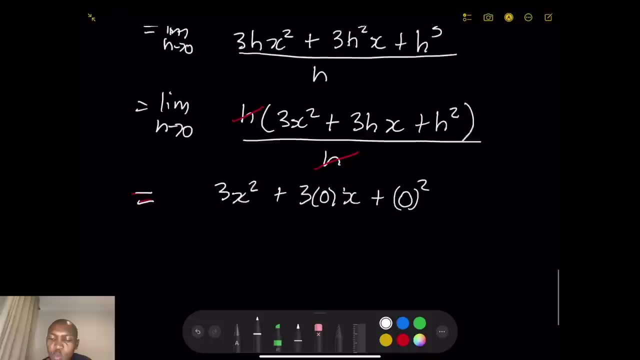 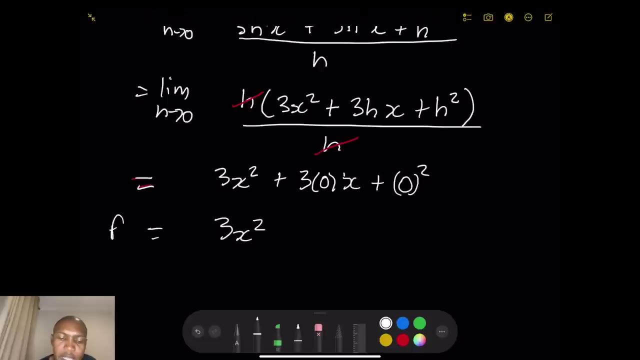 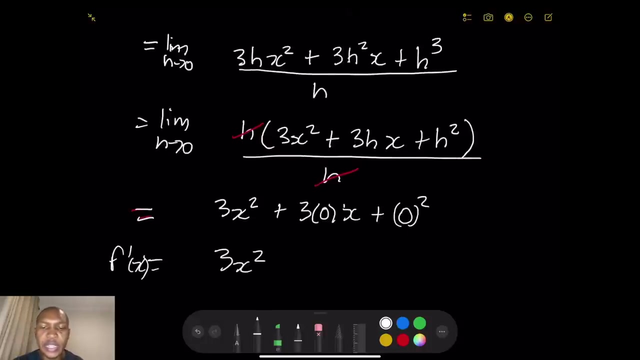 times zero x plus zero, squared, okay. so in this case, what i'm going to do is i'm going to cancel plus three t times dominant over h. right, because we have two h here. so, assuming that we cancel, all right, i think that that's good, right, so i'm going to- yeah, also that filter this over on the. 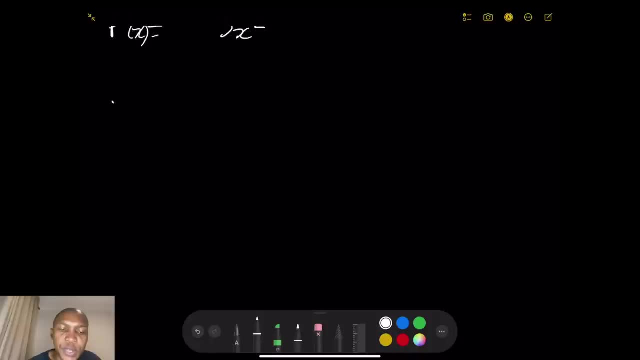 right, playing présent out wars white as well. what does that give us? we ends up with? uh, just simply. Please just get me the derivative from first principles. Now, if f of x is given to be okay, 1 minus 3x squared okay.